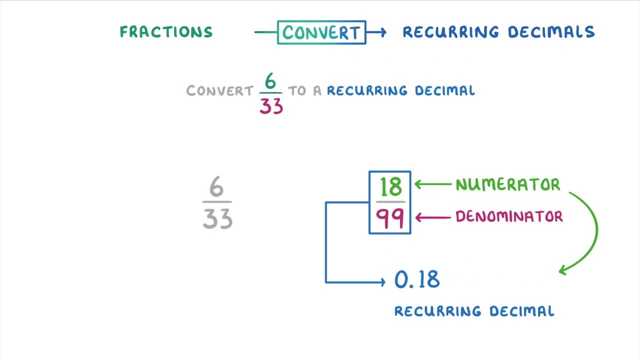 Which we can write as just 0.18,, with dots above the 1 and the 8.. One important thing to know about this rule, though, is that the numerator and the denominator have to have the same number of digits, So in this example, where 18 and 99 both have 2 digits, it all works just fine. 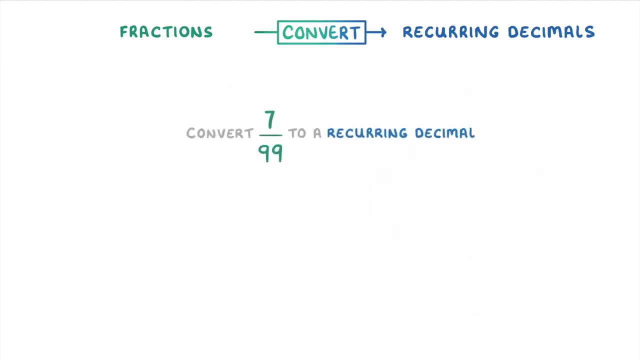 However, if we had a slightly different question and we had to convert 7 over 99 into a recurring decimal, we'd first of all need to make our numerator have 2 digits, Because our denominator has 2 digits. We can do this by adding a 0, to make the 7 become a 0- 7.. 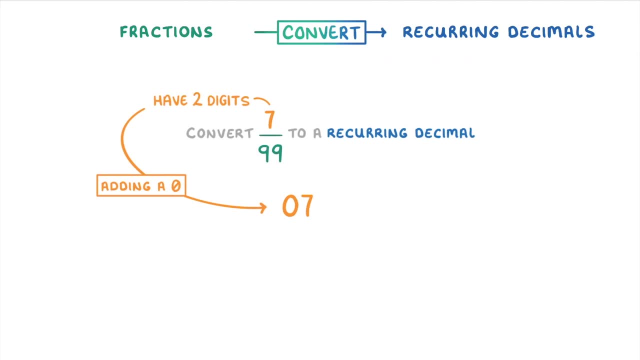 Because this has exactly the same value but now has 2 digits rather than 1. And it will still be over 99.. Now, at first this might look like it won't do anything, But actually it means that in our recurring decimal, the 0 and the 7 are both going to. 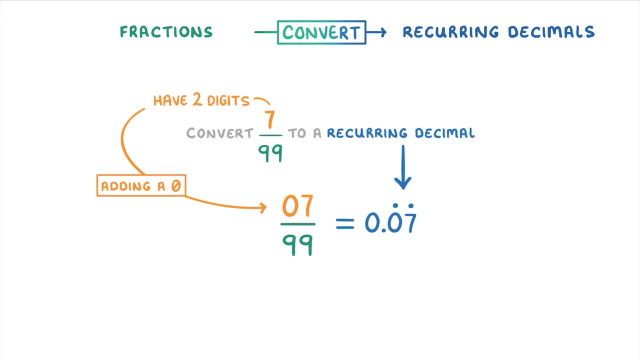 recur. So our answer is 0.07 recurring rather than just 0.7 recurring. Let's try a couple more examples. In this first one we want to convert 2 thirds to a recurring decimal. The first step is to make the denominator a 9.. 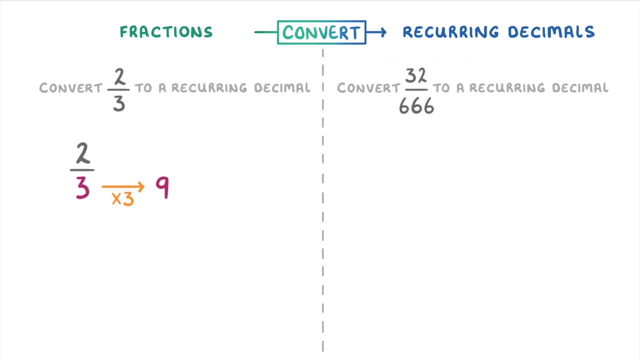 Which we can do by multiplying the 3 by 3.. This means that we also have to multiply the denominator by 3.. We have to multiply the 2 by 3, which is 6.. So we get 6 over 9.. 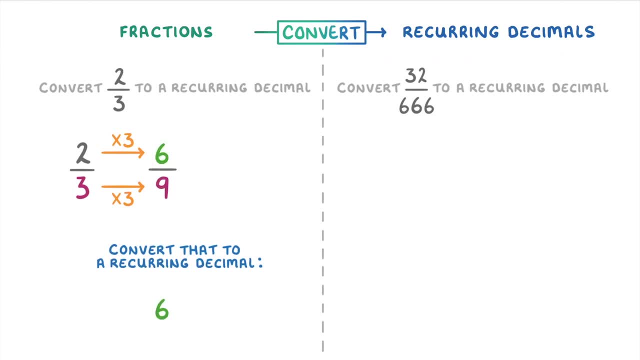 And to convert that to a recurring decimal, we take that 6,, place it after a decimal point and make it recur, Which we show by putting a dot above it. For this second question, we're trying to convert 32 over 666 into a recurring decimal. 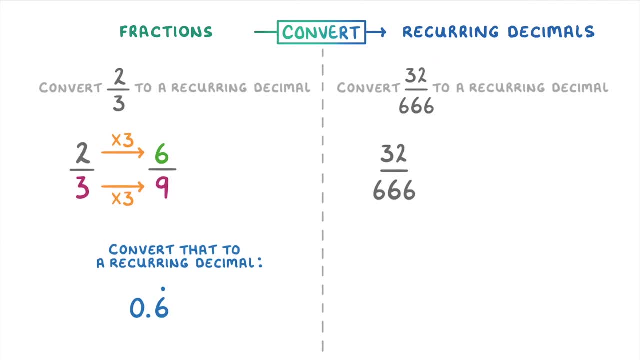 The first step is to convert the 666 into a recurring decimal. The second step is to convert the 666 into 999.. Which we can do by multiplying it by 1.5.. This means that we're also going to have to multiply the 32 by 1.5 as well.